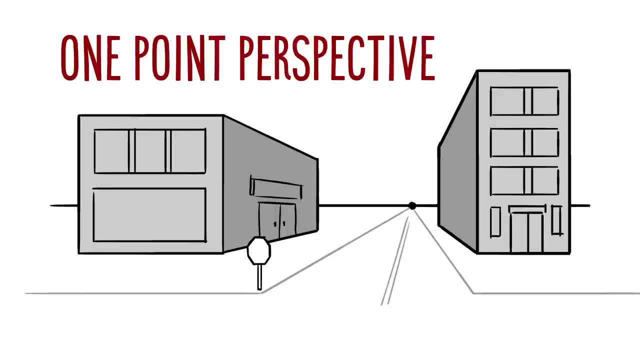 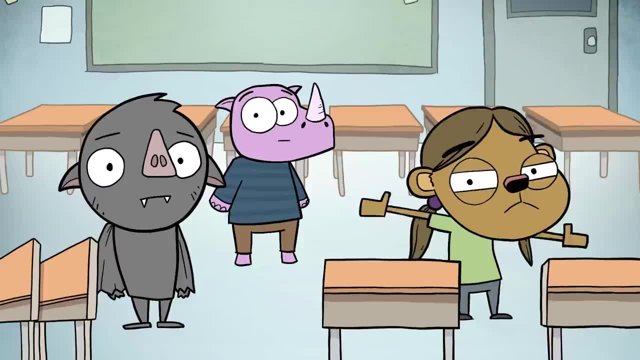 Since there is only one point here, we call it one-point perspective. It's great for simple scenes where you don't want things to feel too flat. Like my desk, Yes, like your desk. Is the DVD talking to you? Whoa? 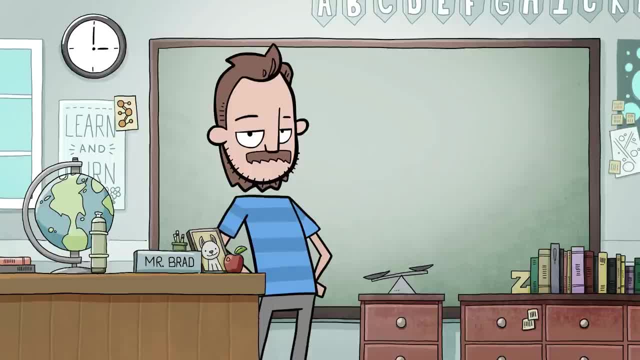 Two-point perspective. has you guessed it? two vanishing points. The second vanishing point is also located along the horizon line. Finding the right spacing between these vanishing points can be a little tricky. If they're too far apart, there isn't much depth to your drawing. 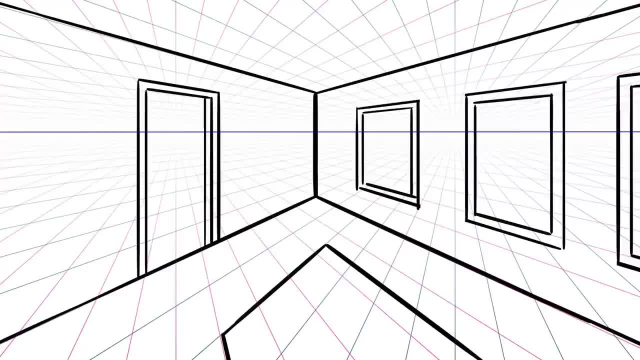 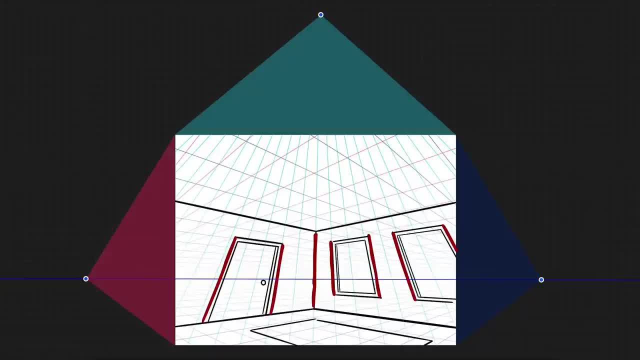 If your vanishing points are too close together, things start to look way too exaggerated. There's also three-point perspective. This is the point that we've been drawing out our vertical lines up and down on, But three-point perspective gives us another point in the sky. 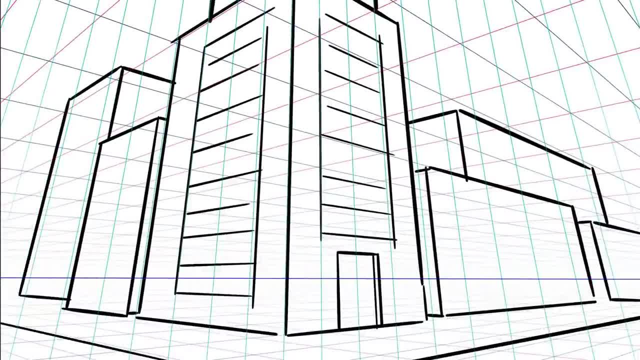 This is great if your character is looking up at something Or if you position that vanishing point just a little higher. it gives you a little more height to your scene. Unlike the first two points, the vanishing point gives you a little more height to your scene. 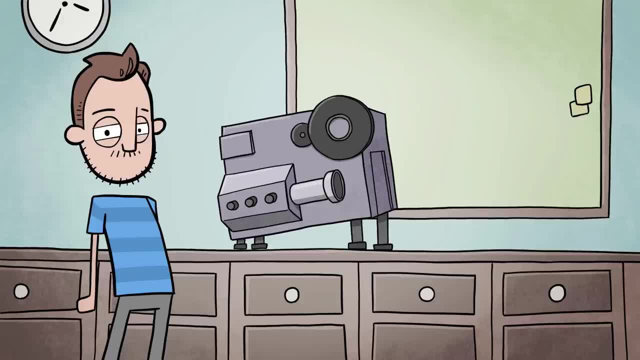 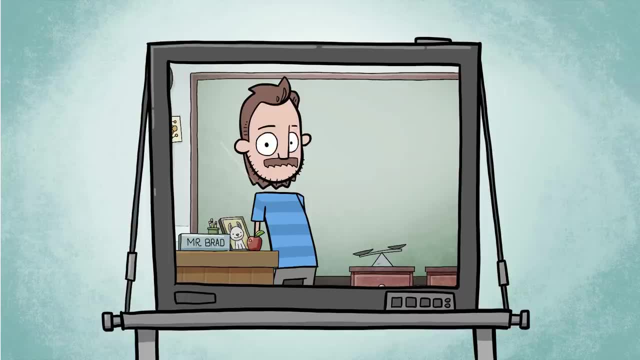 The third point doesn't have to be on your horizon line. Okay, I got it working. No, my lunch. Back to the DVD. Back to the DVD. Let's take a little closer look at the horizon line. The position of the horizon line determines the viewpoint of your drawing For most photos and 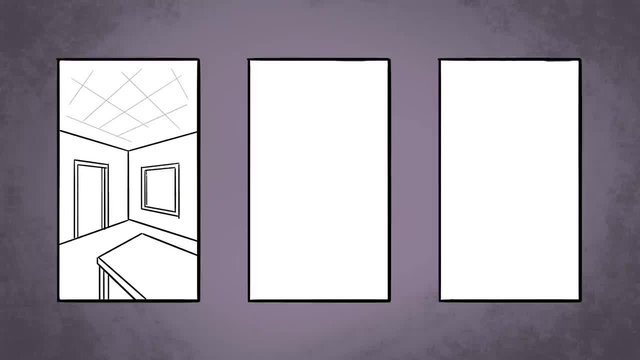 drawings, the horizon line is somewhere in the middle of the page. If you want a top-down view, move the horizon line to the top of the page or even off your canvas completely. If you want a mouse-eye view of the world, put your horizon line along the bottom of the page in 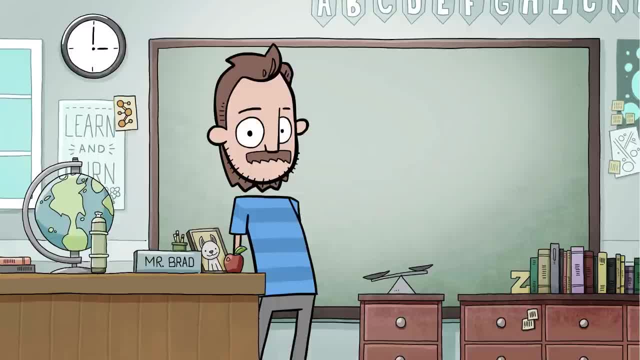 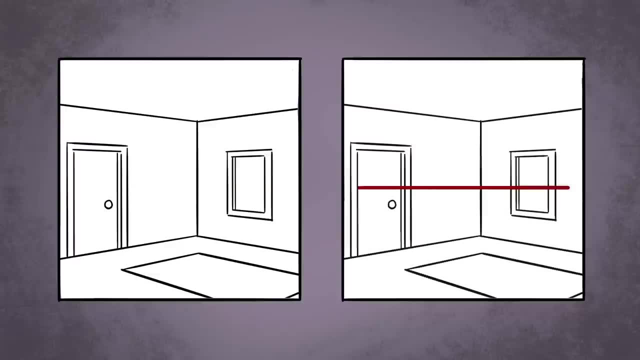 order to look up at your subject. Another technique is to have the horizon line on an angle. You don't see this very often, because we're used to looking at the world when we're standing up, But if you're seeing the world from the eyes of a person who is lying down, 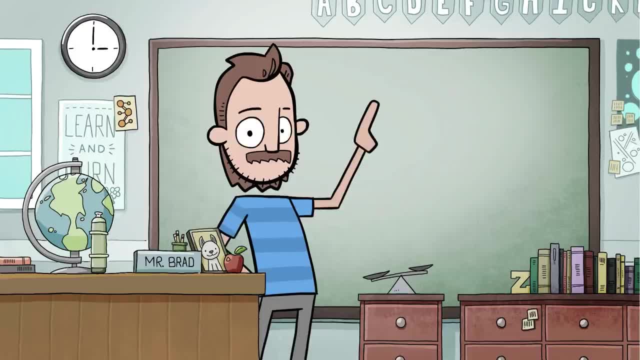 then a sideways horizon line will do the trick. Use this technique sparingly. It may look cool at first to tilt your horizon line, but since it's unusual for the viewer ever to view the world that way, they might end up reading too much into it or just might not connect with the scene because of a 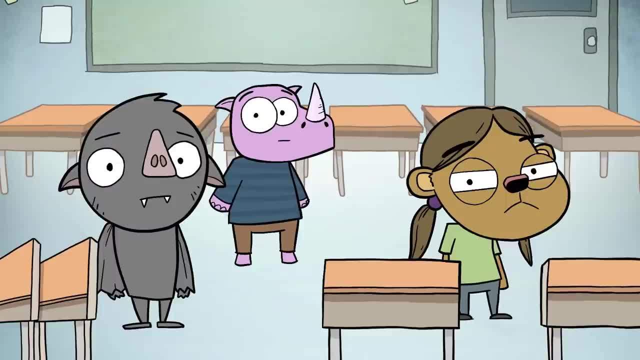 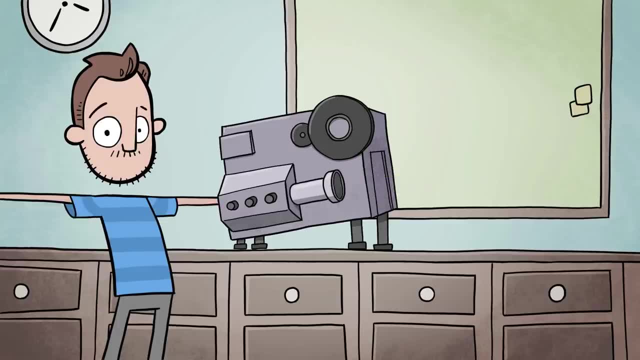 lack of realism, even if all the lines are correct. Check out these really old paintings. They didn't know how to draw a perspective, yet They didn't know how to draw cats either, Or baby humans. Huzzah, It's working. Did you see that? I turned your desk into a real desk. 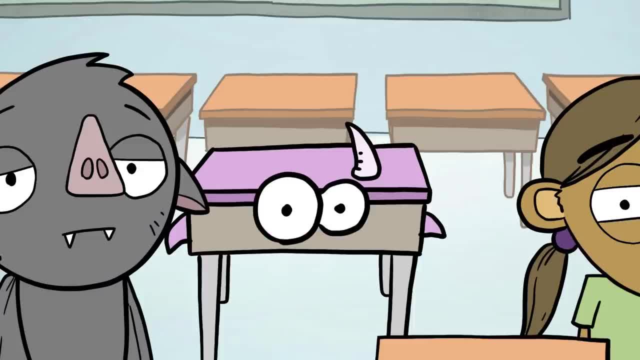 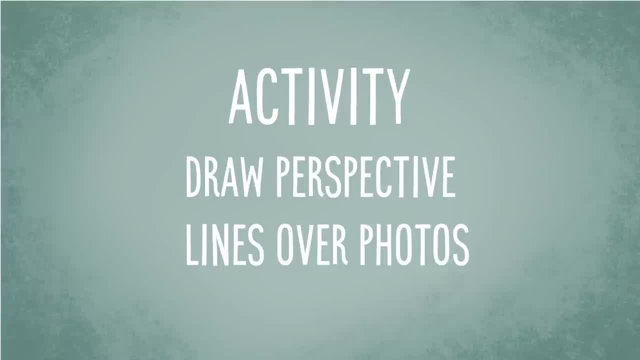 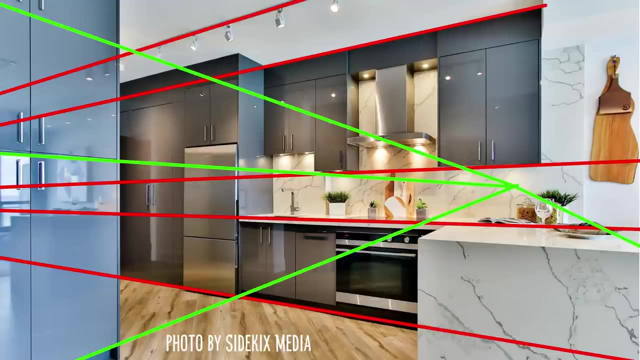 Um no, You turned that rhino kid into a desk. He did what now? Draw perspective lines over photos. If your perspective line looks exaggerated or just kind of off, drawing perspective lines over photos is a great way to figure out what realistic perspective looks like. Doing this a few times will help you see how far apart those 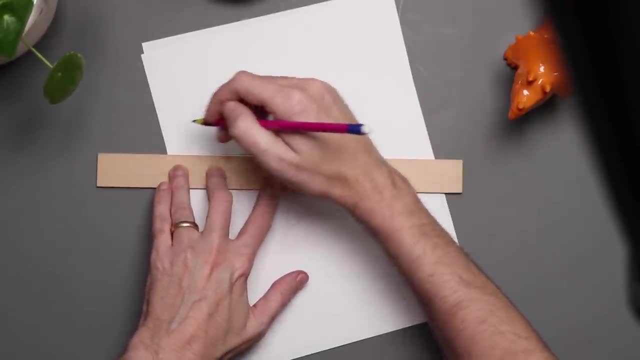 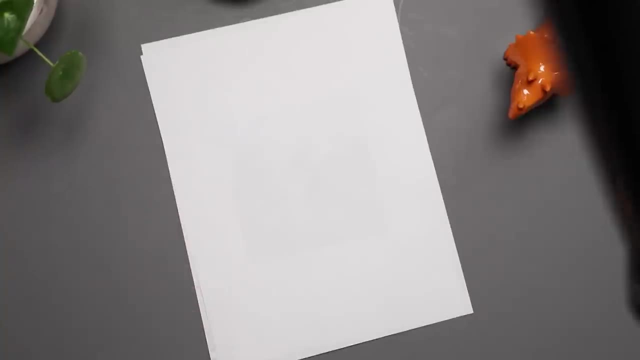 vanishing points should get in order to find the effect that you're looking for. This will also help you find the horizon line if it's not apparent at first. You could do this with pencil and paper, just tracing over a photo that you've printed out or already have, or you could do it. 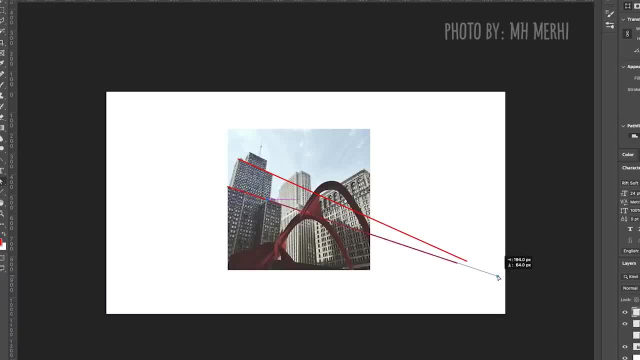 digitally, like I am here. It's going to be easier if you pick out a photo of something man-made- maybe something with buildings or inside of a room- because it's going to give us some nice straight lines to work with. It's going to give us some nice straight lines to. 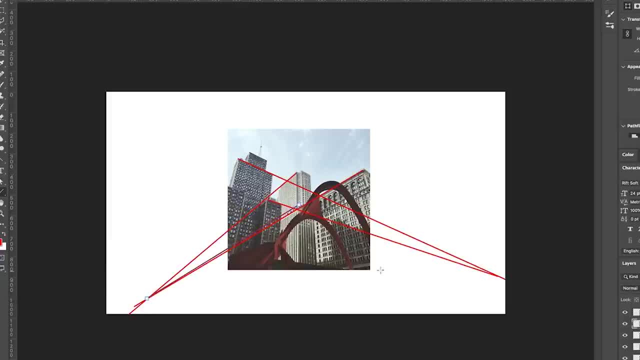 work with. When you're drawing your lines, don't stop drawing. where the line stops, Keep going. It's going to look sloppy at first, That's okay. Then we could jump in and trace out some of the other lines. Where these lines meet is our first vanishing point. 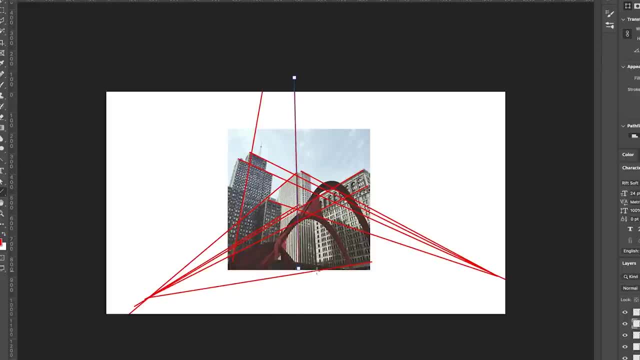 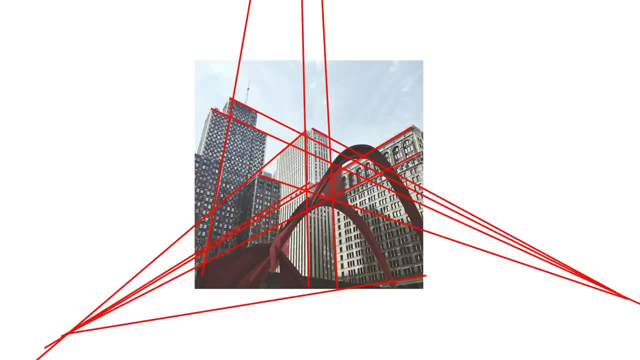 We can then follow back the other lines that are going in the other direction to our second vanishing point. Now that we have the vanishing point, we have all of the basics we need for a good perspective grid. We can add our own lines now to make a real grid. If we wanted to draw a box in this scene. 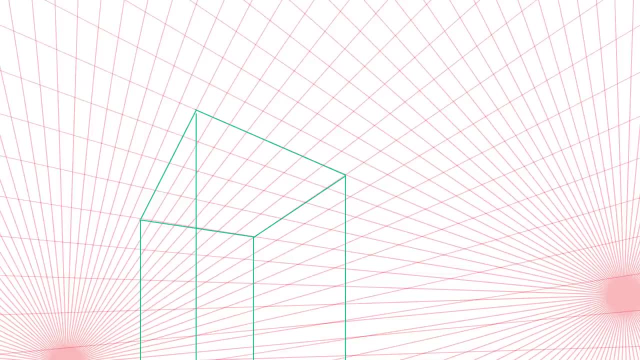 we could use the perspective grid to do that. Or if we wanted to get a feel for where a character would go, we could draw a box roughly the size of that character to figure out the proportions. The next video is going to be all about drawing characters and objects in perspective, so 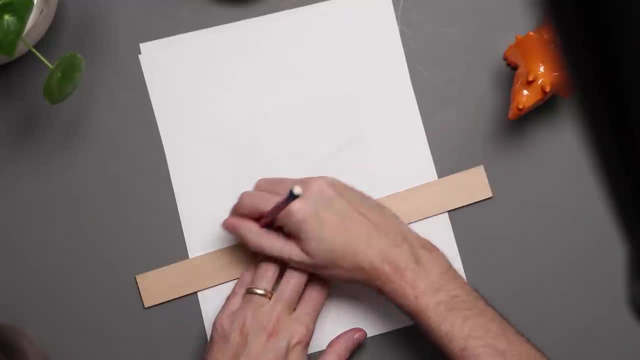 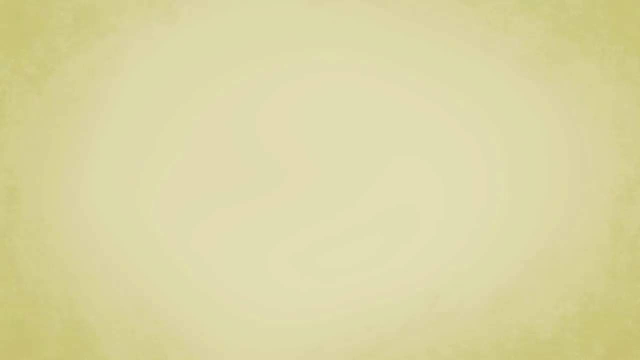 subscribe and ring that bell if you don't want to miss that one. After practicing this a few times, you're going to start to be able to pick out the perspective lines pretty easily and you're instantly going to be able to tell which photos are: 1-point perspective. 2-point perspective. 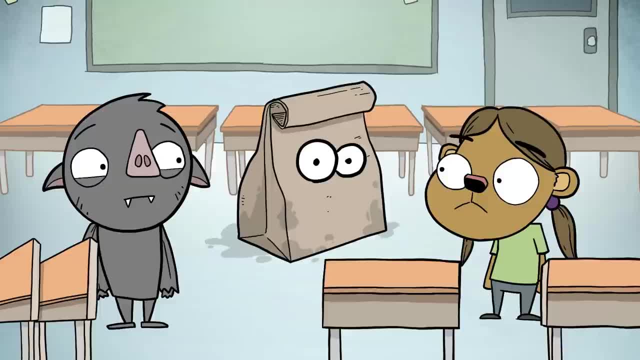 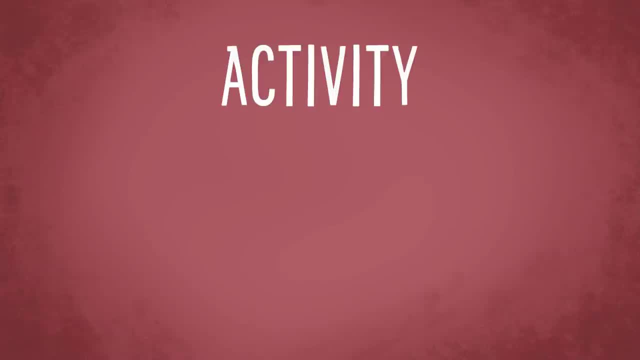 or even 3-point perspective. So let's get started. 1-point perspective: Did that work? Yeah, I think so. No, I think not. At least Mr Brad has a lunch now. He has a. what now Activity? Draw some boxes on a plane. 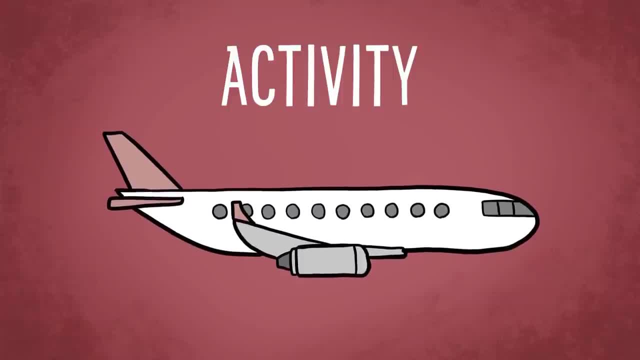 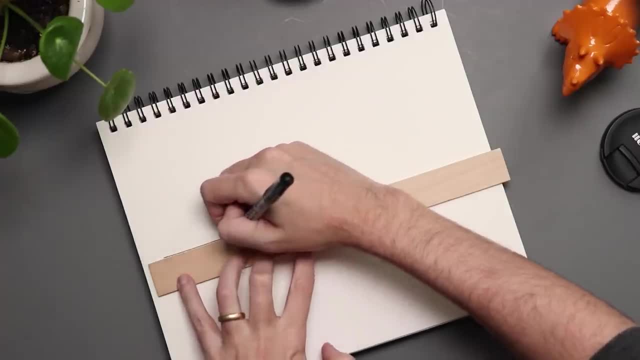 We've been on this plane forever. We should try drawing boxes. Nope, wrong kind of plane. This is going to be easiest if you use 1-point perspective, Create a horizon line and then place your vanishing point anywhere along that line. 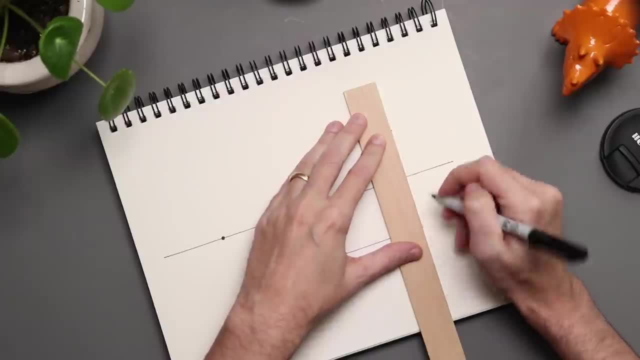 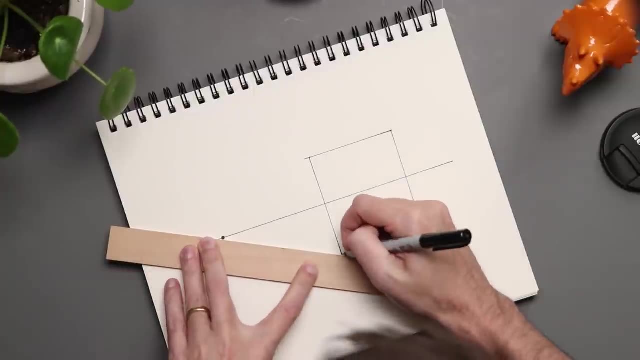 Now let's get to drawing. Start by drawing a box, Just a rectangle, the part of the box that is facing you, And now we're going to create the side of that box. So we're going to draw our lines going back to the vanishing point. 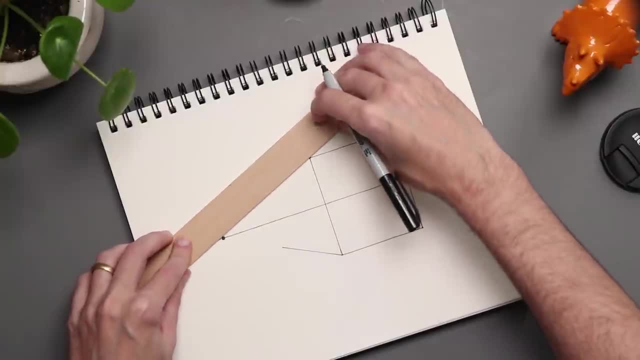 You don't have to draw them all the way back. You can use a ruler. If you draw it digitally, sometimes it's just easier to go all the way back and then erase the parts you don't need. Once these two lines are in place, 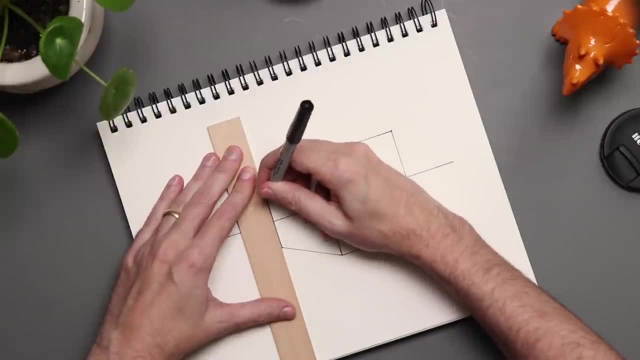 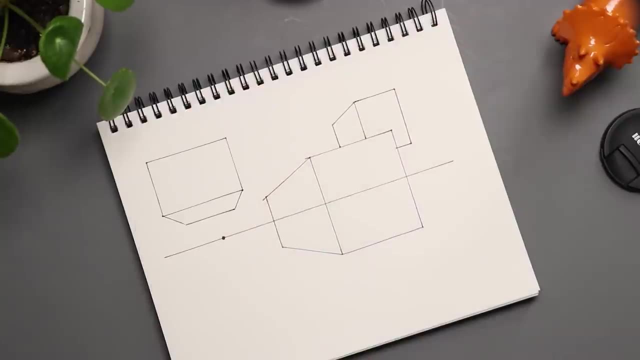 I'm going to add another straight vertical line to show the end of that box. So for this activity I want you to end up with six total boxes. So if this is our first box, let's add one, two, three, four, five to the page. 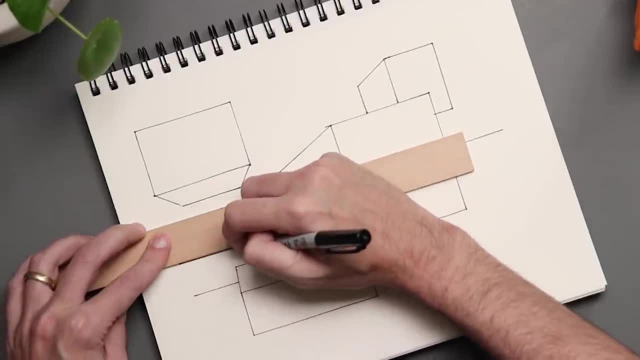 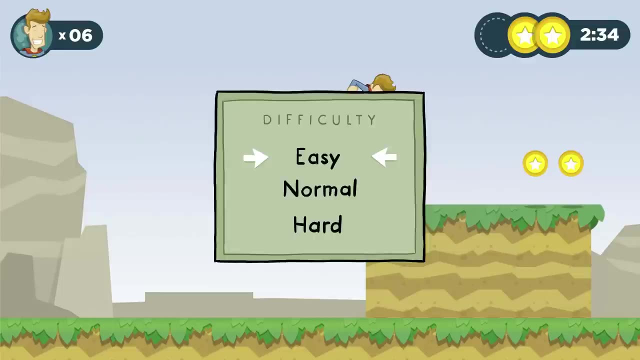 Practice drawing some boxes so that some are going to be in front of the other boxes and some of those boxes are going to be behind other boxes. This is too easy? Okay, then let's shift this from casual mode to normal mode. Try this exercise again. 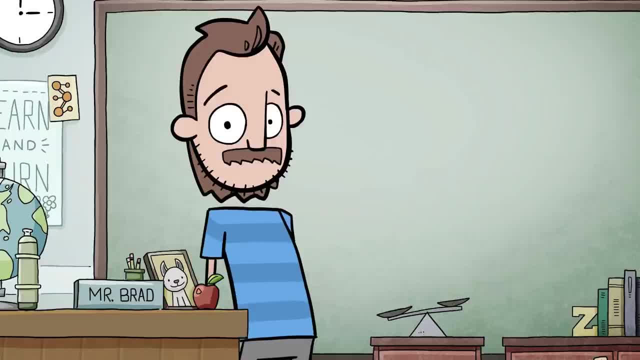 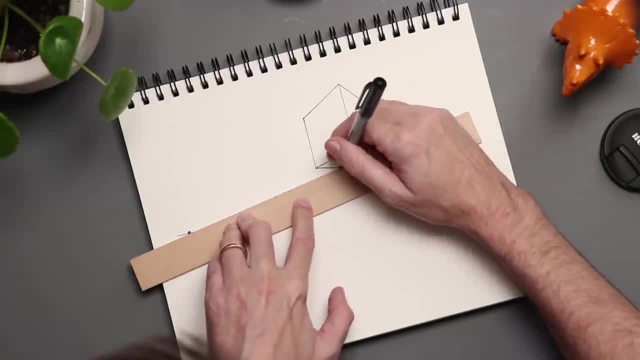 but this time I want you to do it from a 2-point perspective. This time, just draw a vertical line and then each plane of the cube is going to recede to a different vanishing point. And again for this part of the activity, I want you to draw six boxes on your page again. 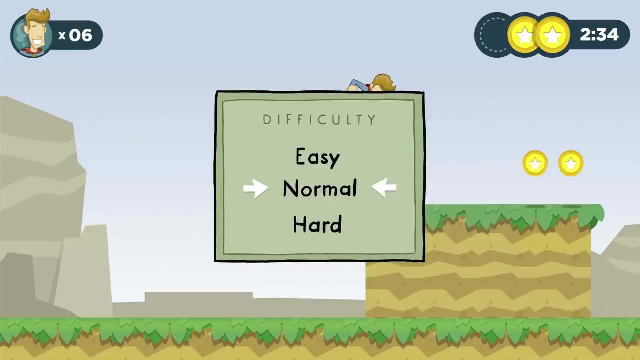 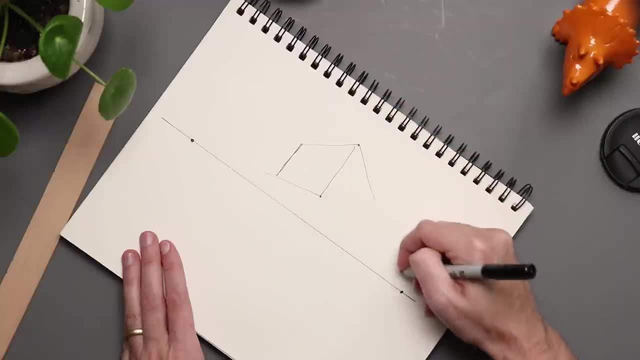 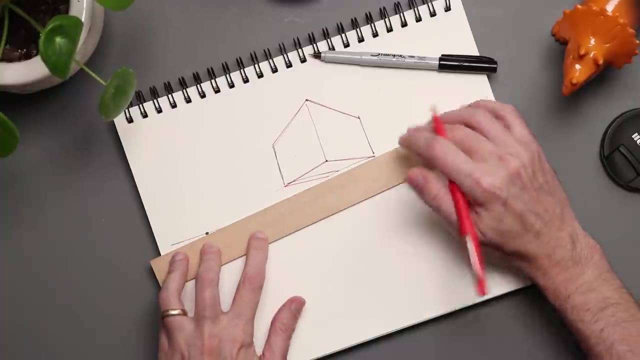 Still not much of a challenge, All right. Well, if you're ready to turn this activity to hard mode, try it without a ruler. This is terrific practice. Practice drawing the lines above the paper or your tablet first. When you're done, you can pull out that ruler and see how close your lines were. 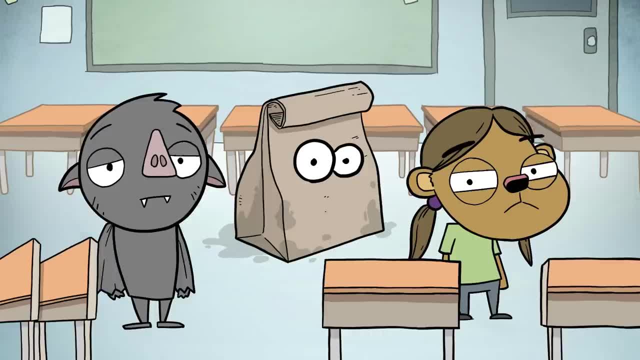 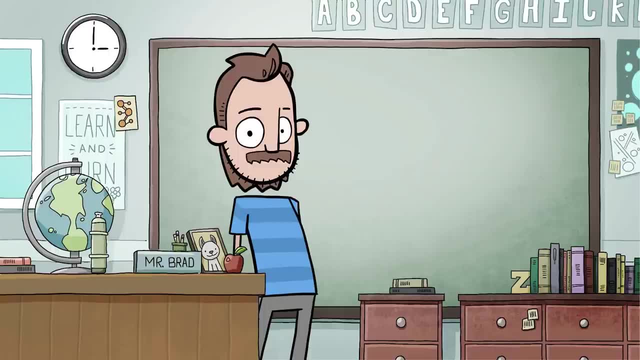 There's actually an entire website with challenges like this on it. Okay, you're right, This is hard mode, I know. Sometimes I'll warm up just by drawing a bunch of boxes freehand, just like this. It helps me understand perspective and you can never get enough practice with this sort of thing. 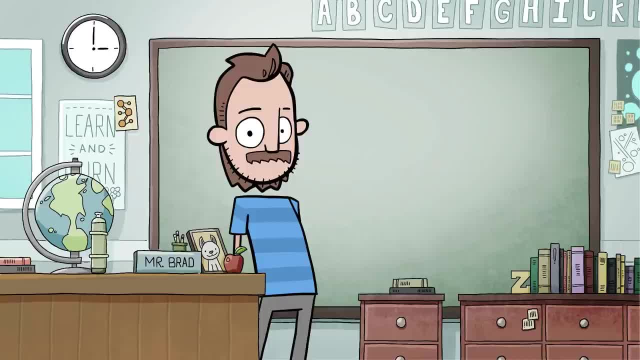 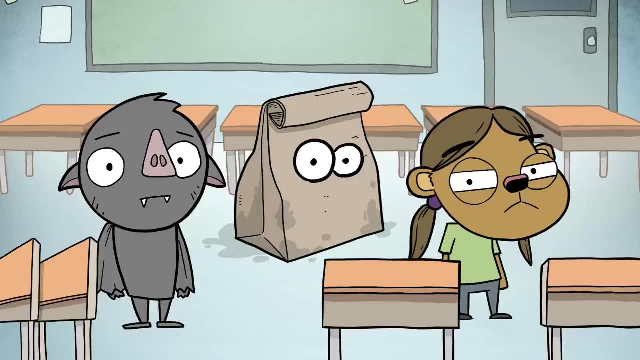 I think I got the hang of this Now that we have a better understanding of perspective. we are going to draw a thing, an actual thing. This thing is a door. Yeah, we can see that. What does it do? It opens and stuff. Let's just draw it. You know the drill by now. 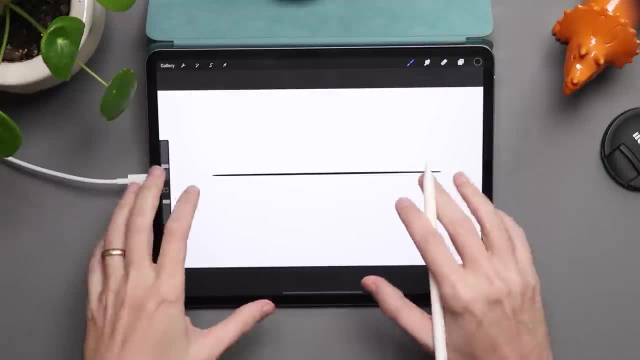 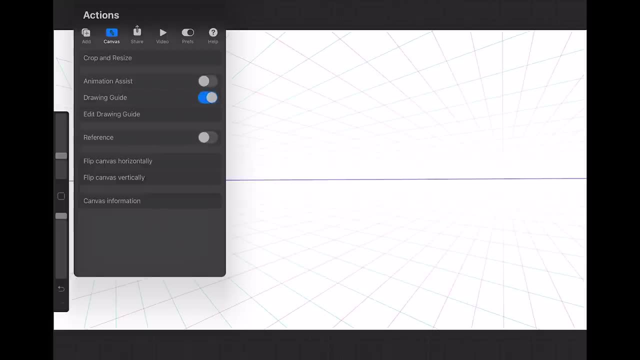 Like everything, we can start with our horizon line and we can pick out our vanishing points, but I am going to cheat. Many drawing apps, like the one I'm using here, which is called Procreate for the iPad, have perspective grids built in that you can go in and modify. 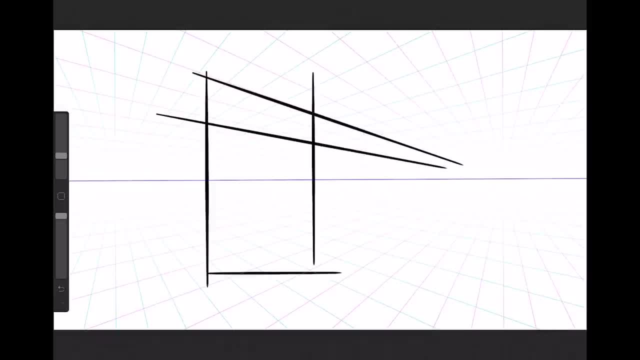 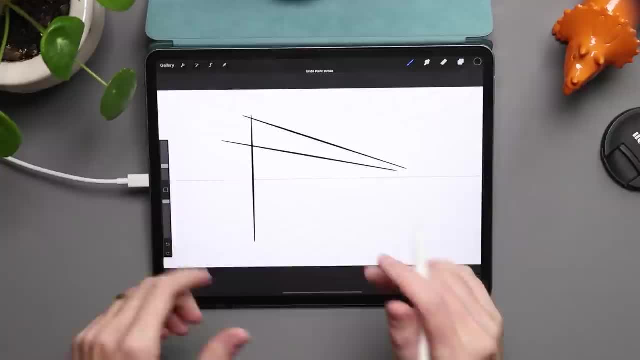 and then you can draw all of your lines already on that perspective grid. If you don't have an app like this, don't worry about it. You can use the same pencil and paper that you've used up to this point, but this oftentimes really speeds things up. 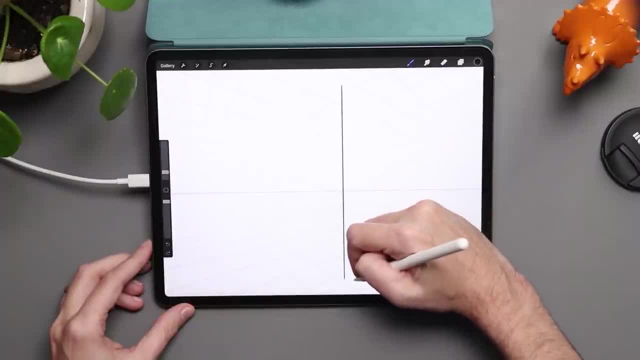 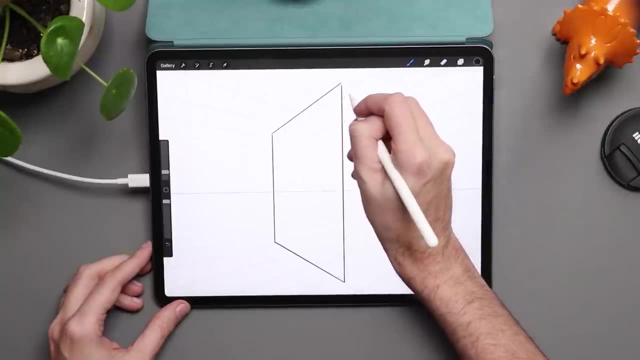 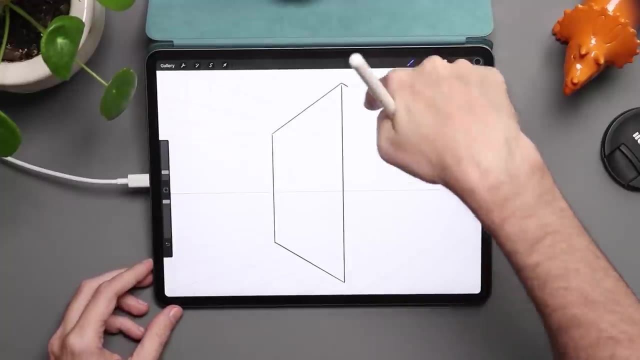 To start our door. we are going to draw a simple box and we're going to draw that in perspective, using our perspective guides, just like this. But a door has a lot more detail than you initially see. For example, that box has some depth, so it's going to go back towards the other vanishing point. 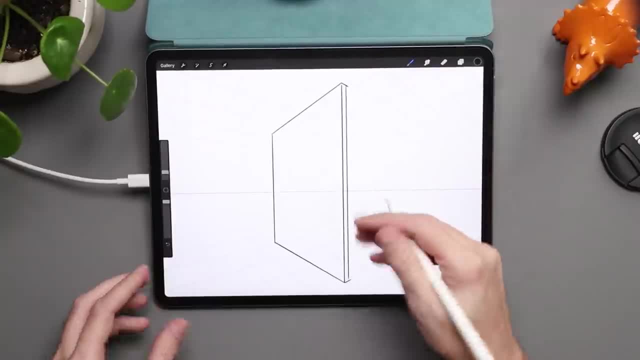 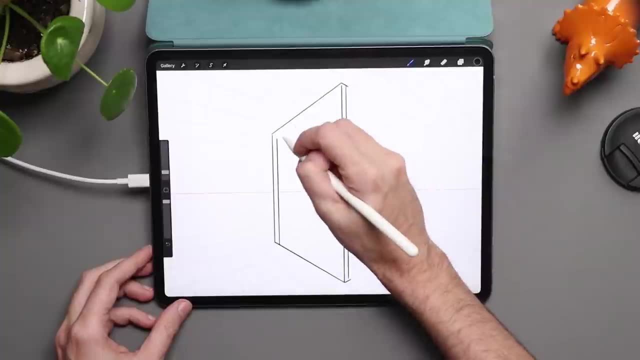 And then I'm going to draw a line over here and now we have a very thin box, But that door also has a frame, so let's draw the frame of that door as well, And that's just going to be an outline around the box, like that. 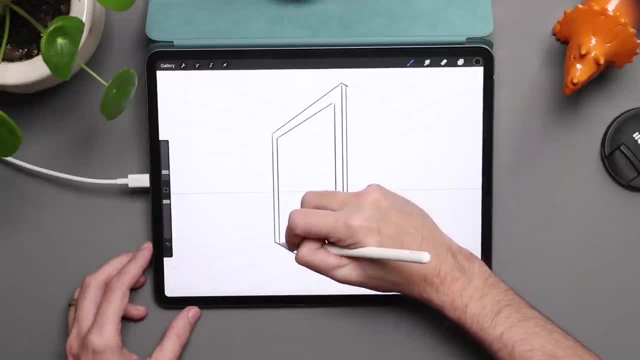 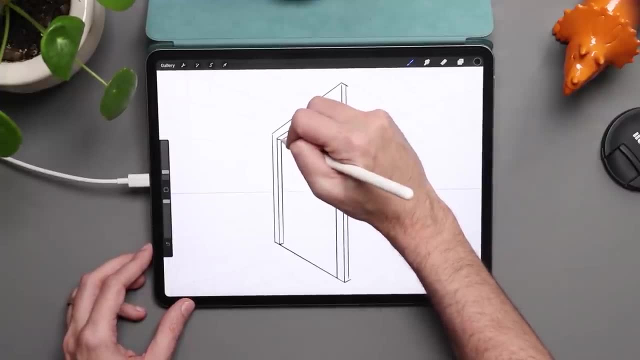 That frame also has some depth. So we're going to come in here and we're going to add that depth. just like that, And by adding depth to your drawings like this, you're not just drawing boxes, but you're drawing the inside of the boxes and the outside of the boxes. 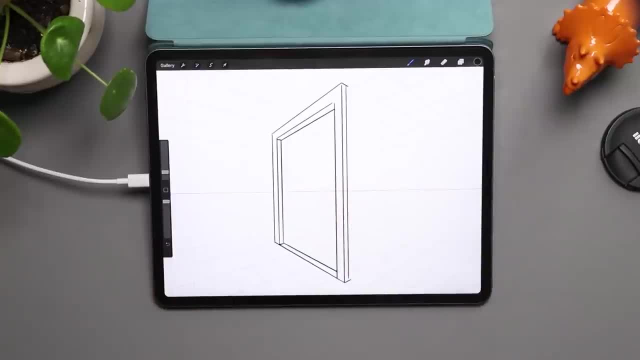 and you're starting to give the entire illustration more depth than it had before. So when we go and add something like a window to this door, if it's just a simple straight window, that's just going to be another box that we're going to be drawing here in perspective. 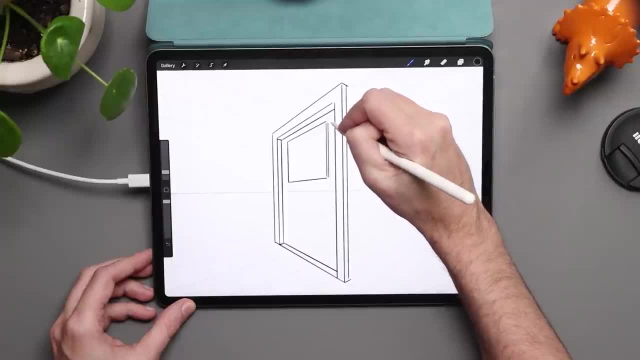 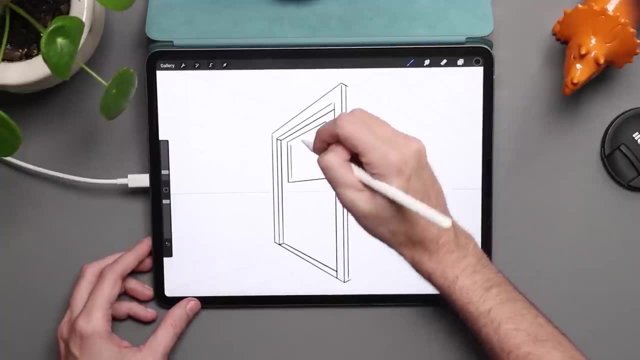 And that stands out a lot. So let's add another line over here to make sure that that has some depth as well. And then, of course, there is the inside outline of that window. So we're going to go in here and we're going to draw that.